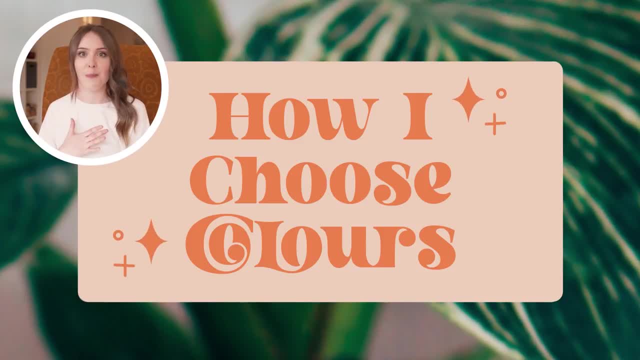 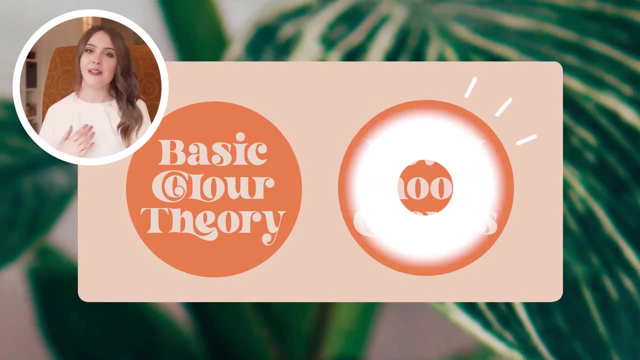 less random, whether you use bold, vibrant colours or muted pastel colours. So the first part of this video is going to be a little bit about colour in general and the second part is going to be about how I choose colours from my own artwork and little tricks I have picked up along the way. 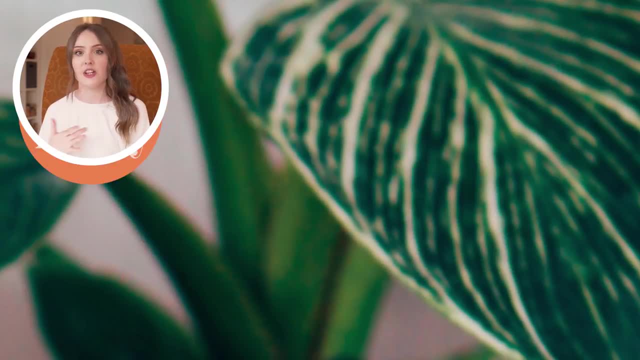 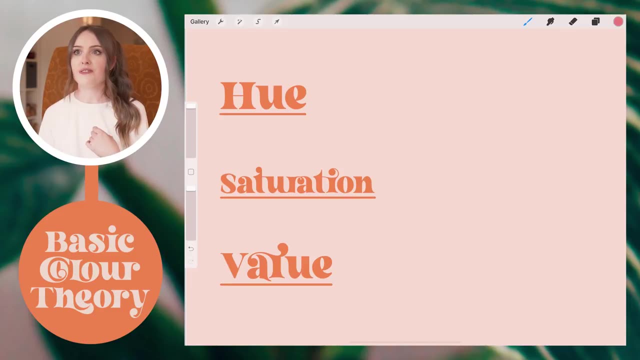 So let's begin with a little bit about basic colour theory. The main terms that you should know about are hue, saturation and value, otherwise known as brightness. Hue refers to the main characteristic of the colour that we see and is basically just the name that you would use to describe the colour. 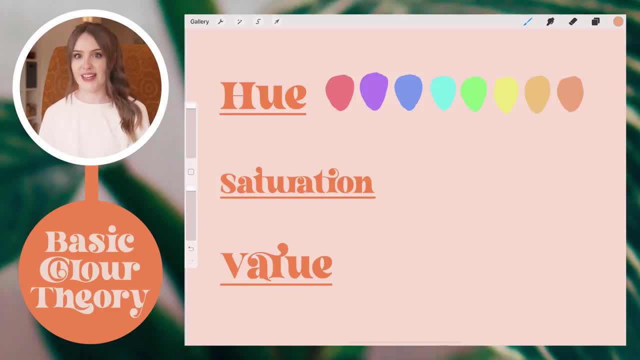 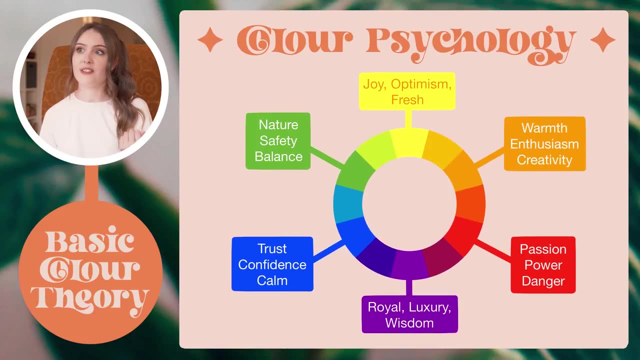 So is it purple, Is it blue, Is it green? You get the gist. Different hues have different psychological ties and it's important to know which colours you choose And this can really drive the emotion of the scene. So, for instance, red is associated with danger and passion and blue is associated with calmness. 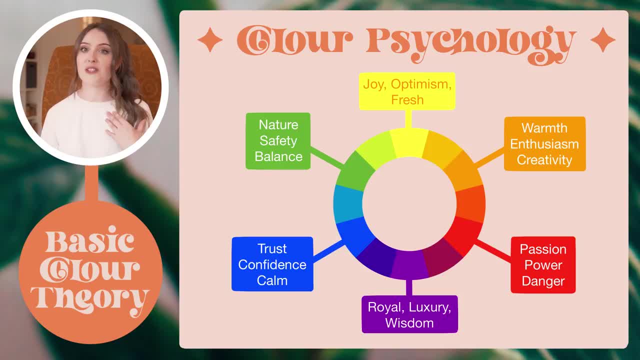 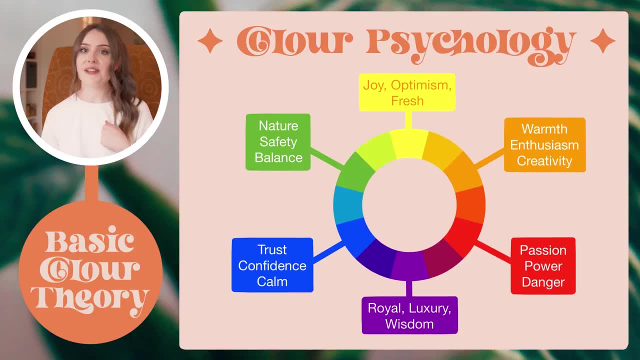 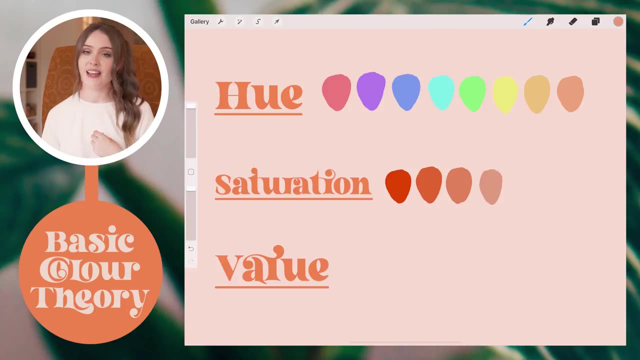 and trust, but I'm sure you're already familiar with most of these. So when you're choosing your colours, you can use these traits to elicit a specific response from the viewer. So now let's touch on saturation. Saturation refers to how pure or greyed down a colour is, So more saturated colours are. 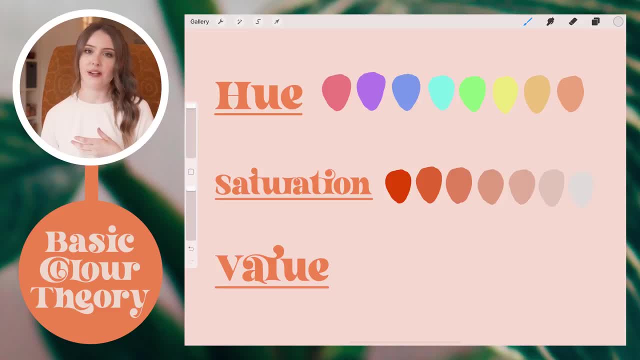 usually bright and vibrant, whereas desaturated colours are usually dulled down and a little bit greyer. And finally, value refers to the lightness or darkness of a colour. Value determines the contrast in your drawings, and it can also be used to strategically make certain elements of your composition stand out. 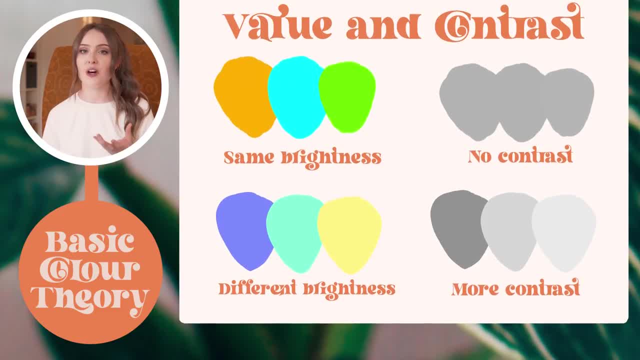 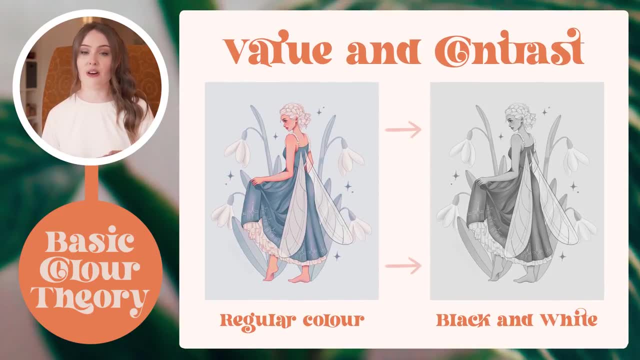 In most cases, when you're building a composition, you want the contrast to be balanced. You can actually check your values by making your drawing black and white, and this should reveal whether or not there is enough contrast in your illustration and if there are certain areas where the values need tweaking. 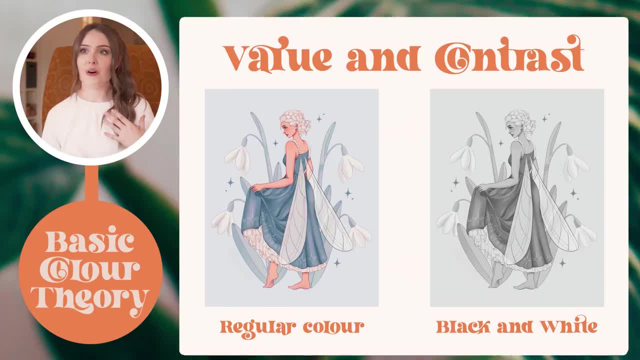 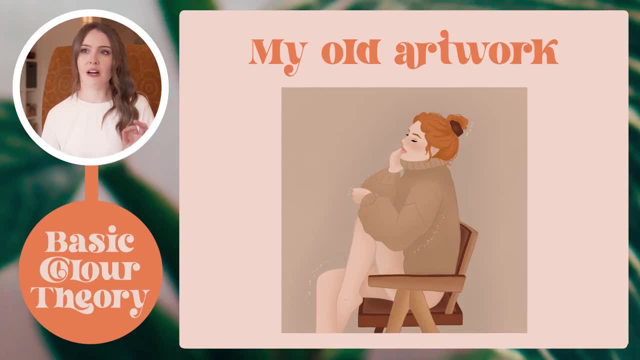 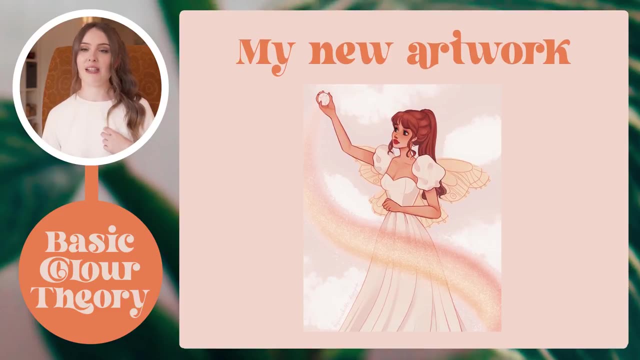 A mistake that I made when I first started making art was by being afraid to use more saturated and brighter colours. I was often adding a lot of darkness to the colours in my early work and it gave it a very muddy appearance. Adding a bit more saturation and brightness can really make your work more crisp and visually. 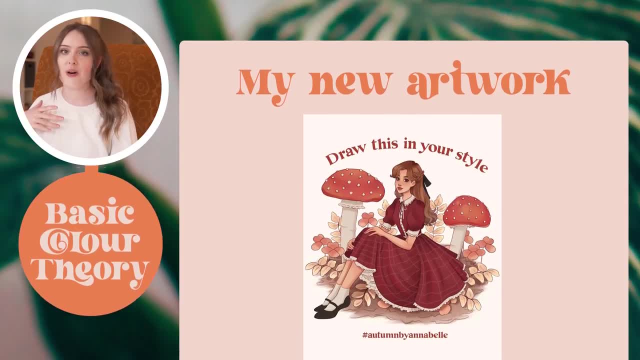 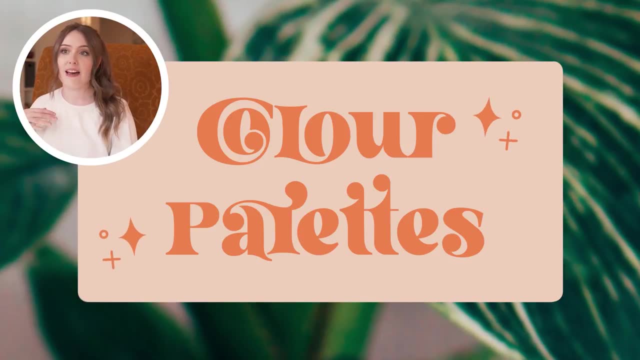 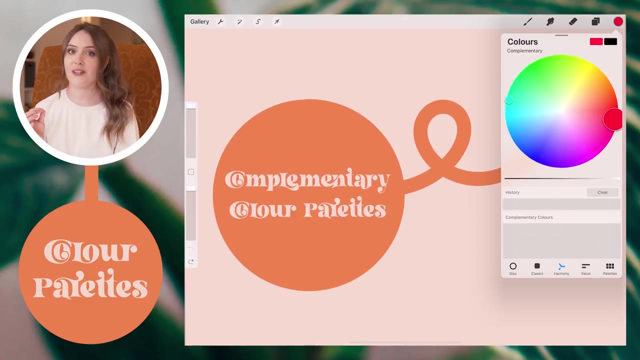 appealing. Knowing about these concepts is helpful for when you are building a colour palette. So two common types of colour palettes that you'll often see in artwork are complementary and analogous colour palettes. First let's talk about complementary colour palettes. Complementary colour palettes use colours that are opposite from one another in the 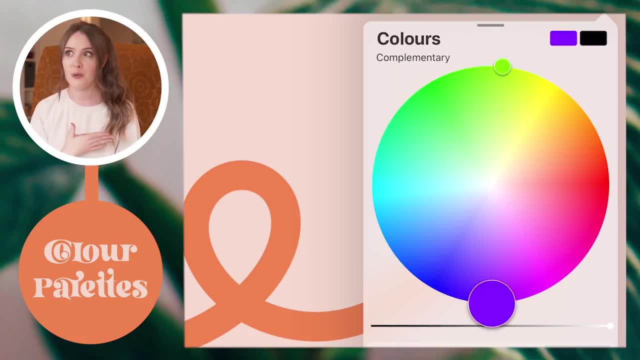 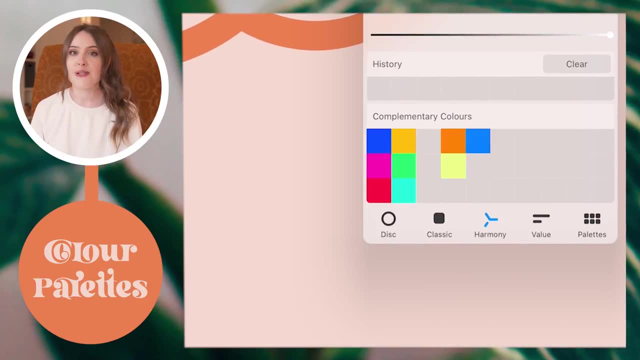 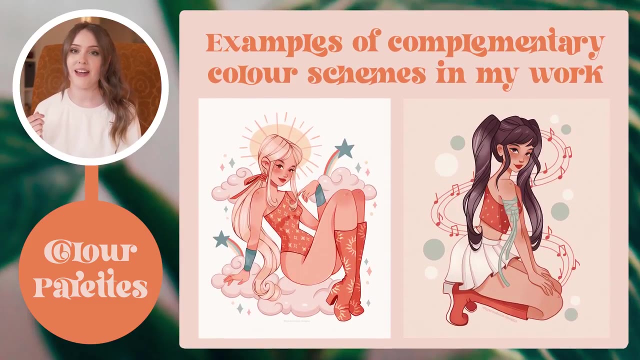 colour wheel. For example, you have blue and orange and you also have green and red. These colours complement each other quite nicely and can make different elements of your composition pop by creating an interesting colour contrast. So here are a couple of examples of how I use complementary colour schemes in my work. 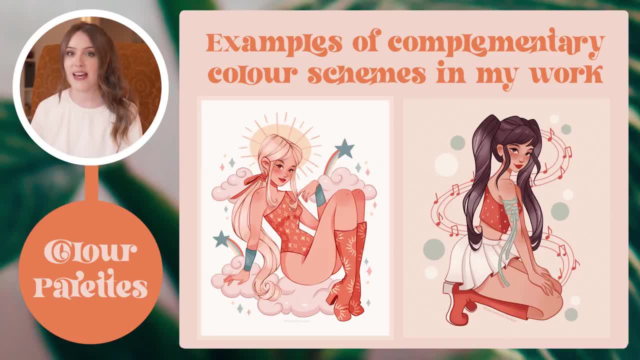 So in this first one you can see that I am using orange and blue, and in the second one you can see that I am using green and red. Complementary colours can be quite overpowering, so you might be able to see that in my work I use one colour as the main colour throughout the piece and the other colour as an accent. 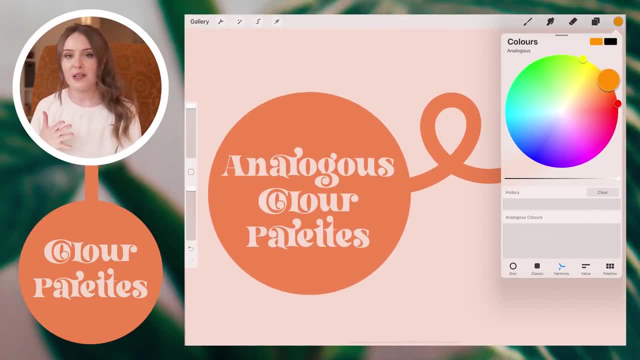 colour. So now let's talk about analogous colour palettes. Analogous colour palettes use colour palettes that are opposite from one another in the colour wheel, So you can use colours that lie next to each other in the colour palette instead of across. 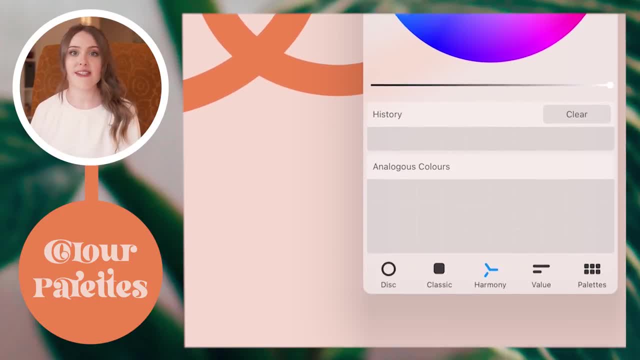 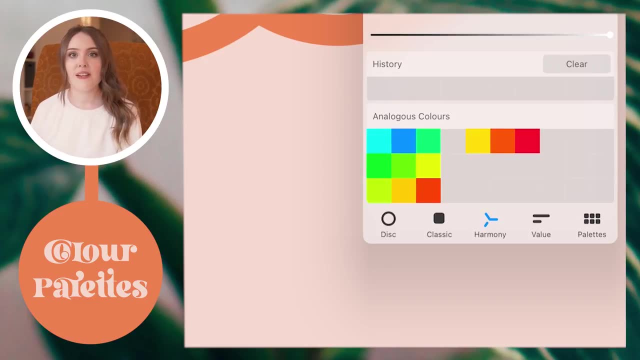 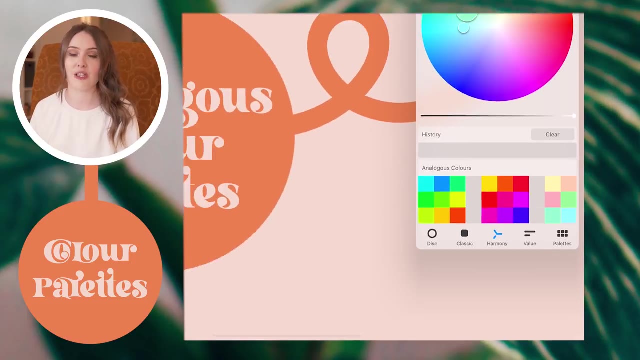 from one another. These colours will usually share quite a few similarities and they're often used to create scenes that are very comfortable to the eye. When you're using an analogous colour palette, you will often use value to create contrast, because you're not using like a range of different colours to create that colour contrast. 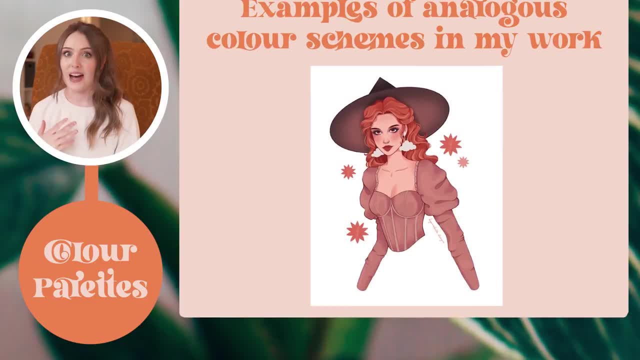 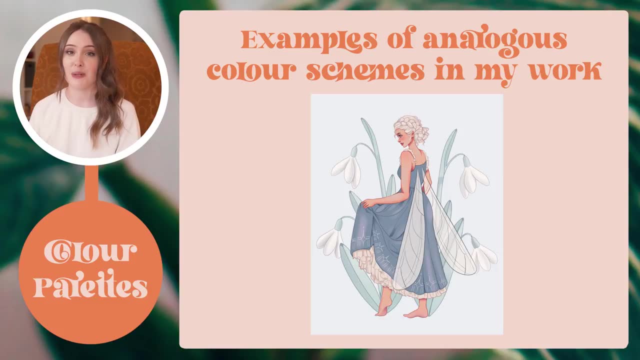 that we talked about earlier. So here are a couple of examples of how I've used analogous colour palettes in my work and you can see on this one I am using different colours and different shades of blue, and in this one I am using different shades of green. 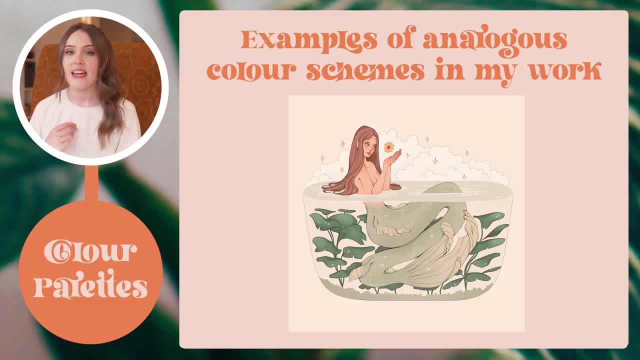 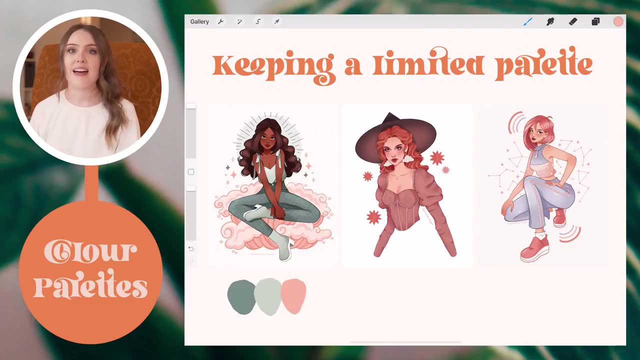 One technique I use to simplify my colour selecting process is by keeping a limited colour palette. Limiting the number of colours that you use in your work eliminates chaos and also makes your work look more confident and well thought out. I try to stick to two to three different hues, not including the skin or the hair colour. 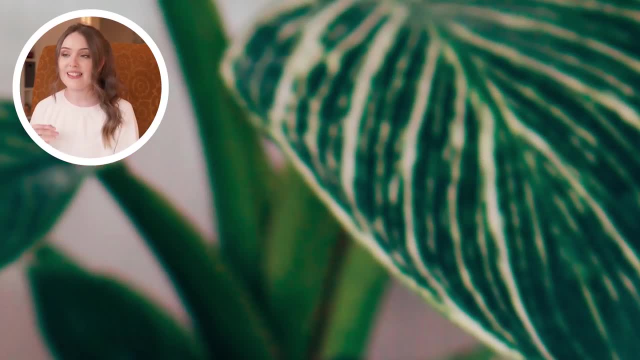 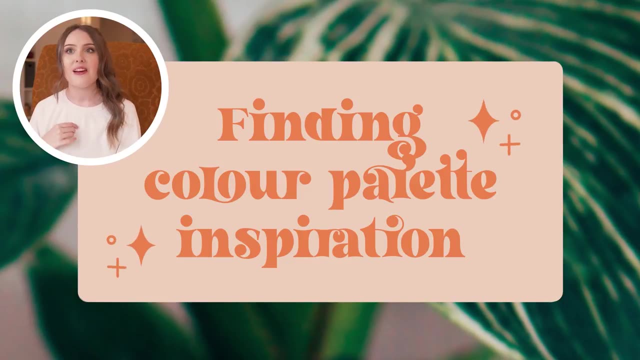 of the character. Now that we've covered the basics of colour palettes, Let's talk about colour preferences and how to find your favourite colours. I think everybody already has a general idea of the colours that they tend to gravitate towards. You can usually tell what's aesthetically pleasing to you by looking at things like 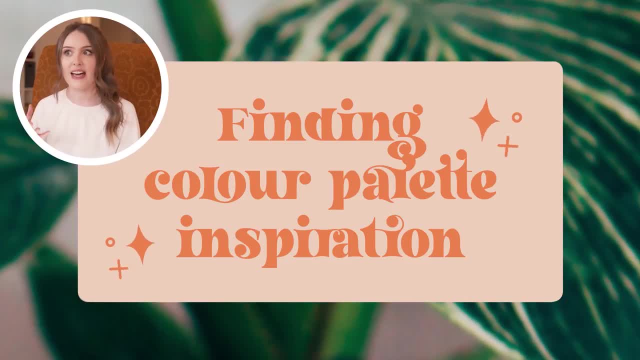 your fashion sense, your interior and even your favourite artists. But if you are feeling a little bit stuck about which colours you want to include in your illustration, or maybe you're bored of using the same colours and want to spice things up, A great place to start is with Pinterest. 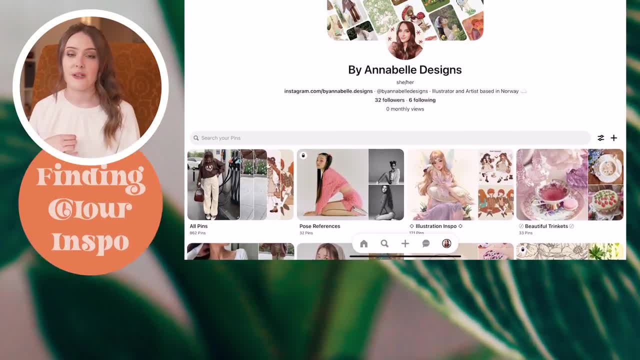 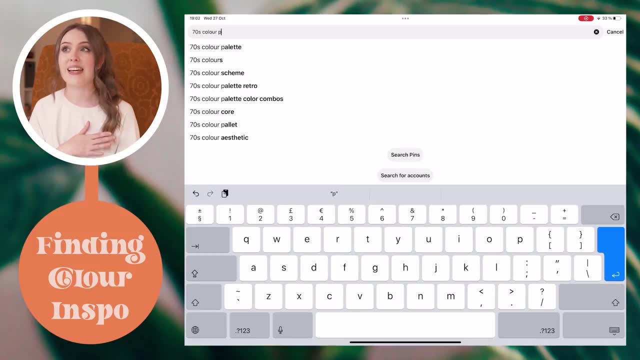 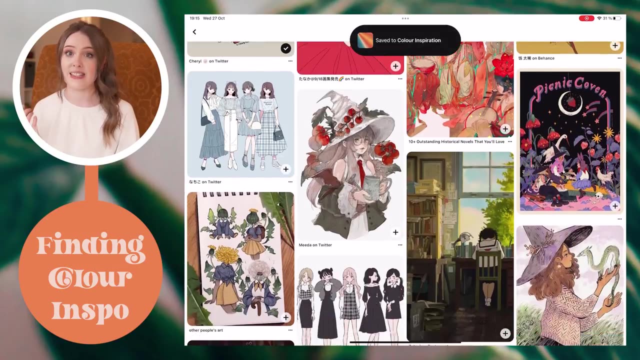 At the beginning, when I was trying to figure out which colours I wanted to include in my illustrations, I created a Pinterest board called Colour Inspiration and here I pinned basically anything that I like the colour of. That could be art, interior, fashion. I mean literally anything, as long as it was aesthetically. 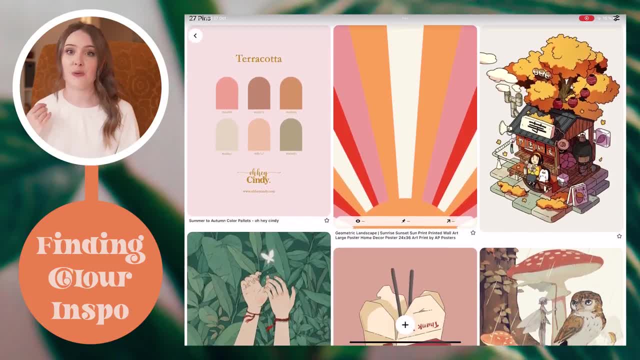 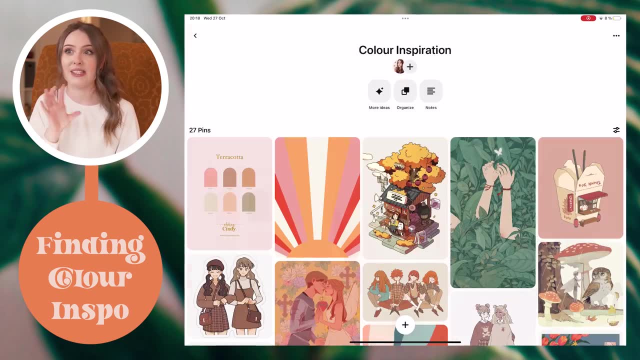 pleasing to me, So I added all of these images into my board and when my Pinterest board had more than 15 to 20 images inside, I zoomed out so that I could see all of the pins together at a glance, and I took a screenshot. 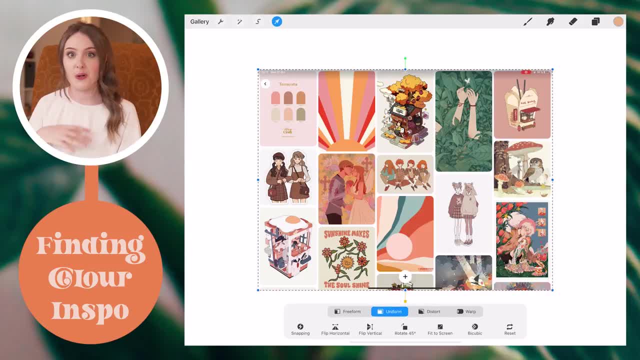 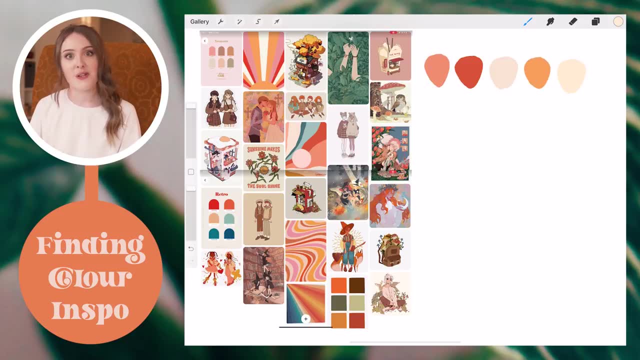 From here. I imported this screenshot into Procreate and used the colour picker tool to select some of my favourite colours from this board and created a new colour palette. As time's gone on, I have refined this colour palette with a lot of trial and error and 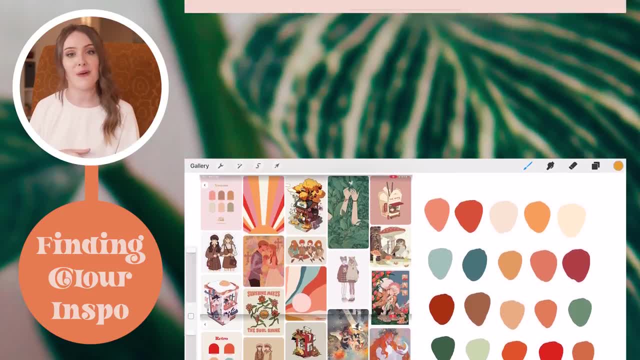 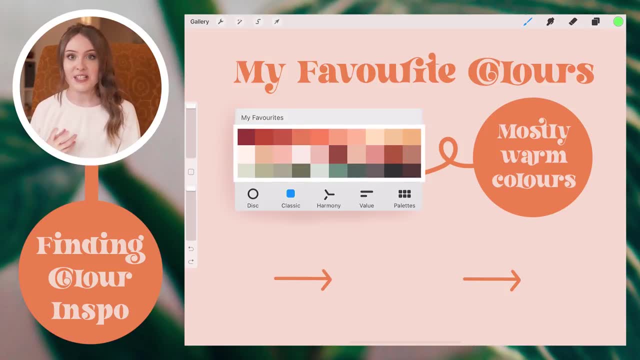 I've discovered which colours I enjoy using the most in my work. Personally, I like to use a lot of warm colours over cool colours. You'll see a lot of different colours in my work. You'll see a lot of pinks and oranges in my work, because that is just what I gravitate. 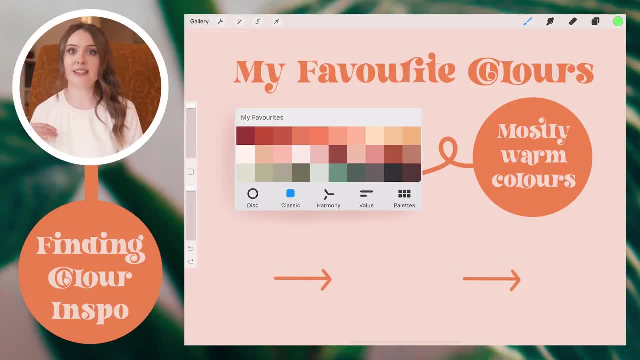 towards. When I'm creating my warm toned colour palettes, I'm often thinking about how I can manipulate colours to make everything more cohesive. So if I wanted to bring in, like a blue or a green, to a pink or a peach dominated drawing. 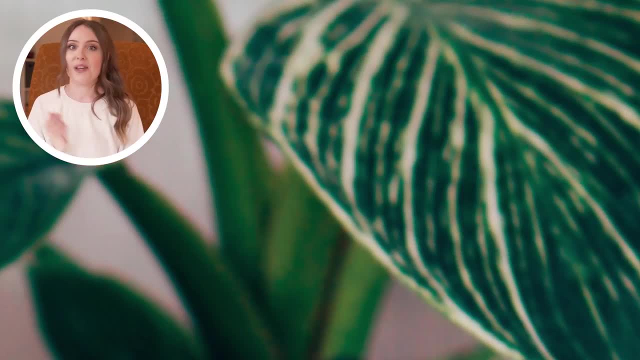 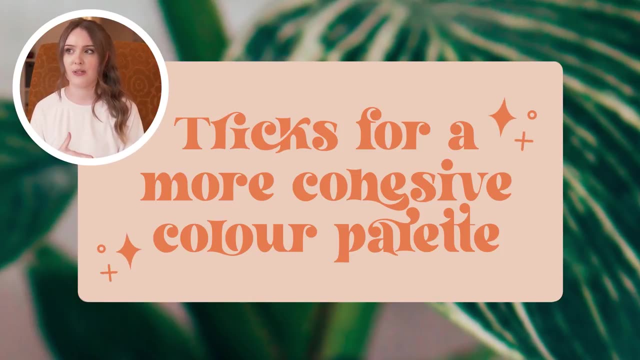 I could do this and keep it on theme and easy on the eyes. So these are a few tricks that I have learned to make my colour palettes more cohesive, And I think this works regardless of whether you're using cool or warm toned colours. 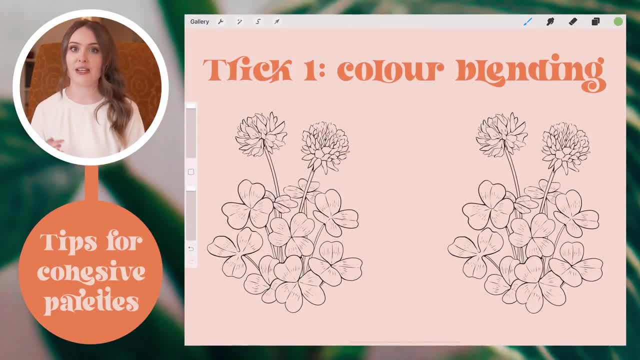 Firstly, when you're choosing your palette, you can blend your colours either with the background or the skin colour to give them a similar base. hue, Say, I have a pink background and I want to add green plants to my illustration. To make this green colour work well with the background, I can add the green on top of. 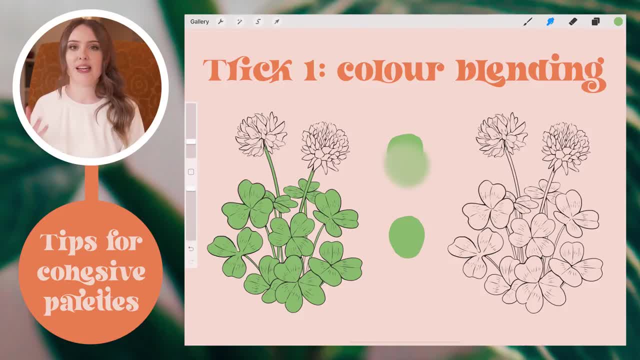 the pink and either use a blending brush to mix these two colours together, or I can simply lower the opacity of the green layer. You can then use the colour picker tool, and this should create a new green that is a little bit more cohesive or more fitting with the background or the skin colour. 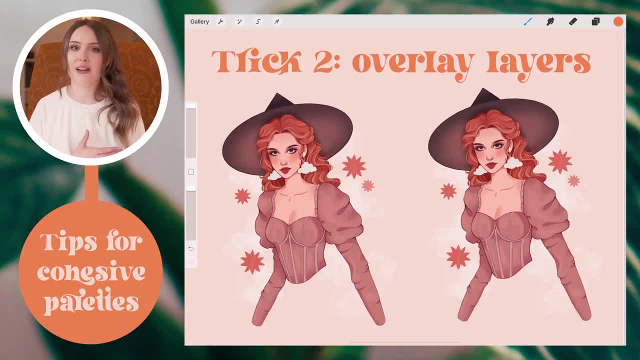 Another way you can make your colour palette more cohesive is by creating a low opacity overlay layer on top of your chosen colours. For example, if I want all of the colours to have a warm undertone, I can create a new layer on top of everything, set it to an overlay blend mode and fill the entire canvas with. 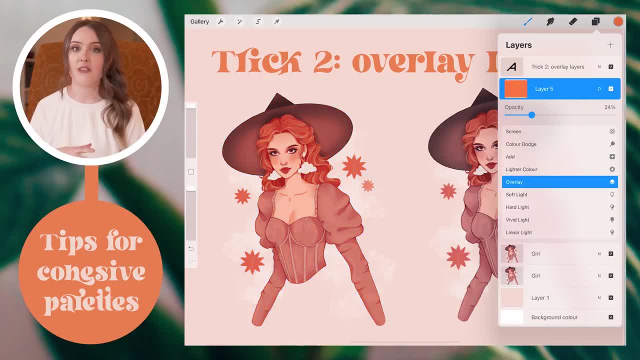 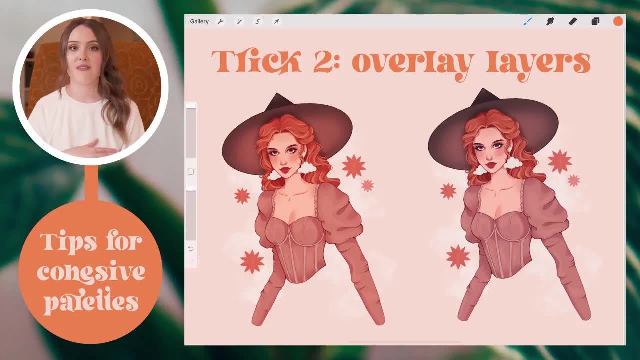 an orange colour. I can then decrease the opacity and you'll see that all the colours within the illustrations begin to take on a warmer appearance. You can do the same thing with a blue colour, so you could fill the whole canvas with blue and, as you can imagine, it would make the colours take on a cooler appearance. 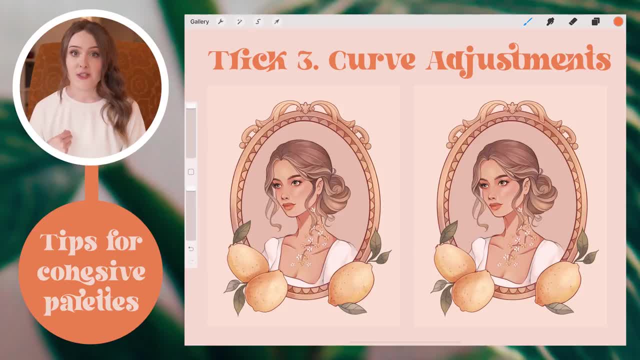 And finally, the last trick that I use comes at the end of my illustration process, and that is by adjusting the curves. First, you want to make sure that everything is on one layer, and then, in Procreate, you can go to the adjustments menu and select curves. 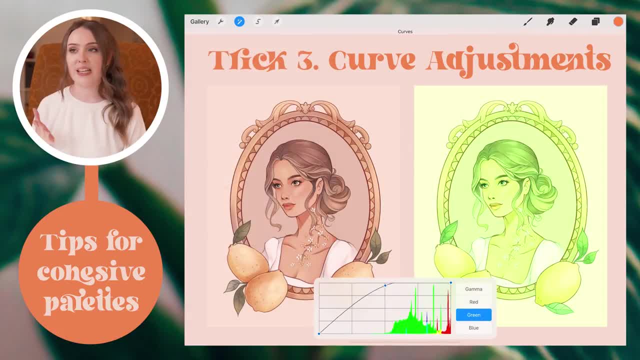 This tool allows you to make different colour adjustments by pulling the reds, blues and greens up and down, Depending on the look you want to achieve. For my work, I usually pull up the red midtones to increase the overall warmth of an illustration. 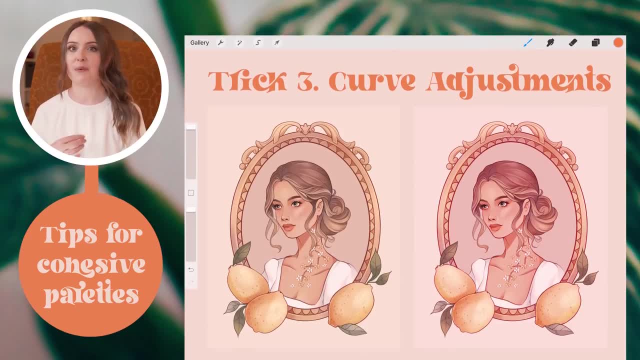 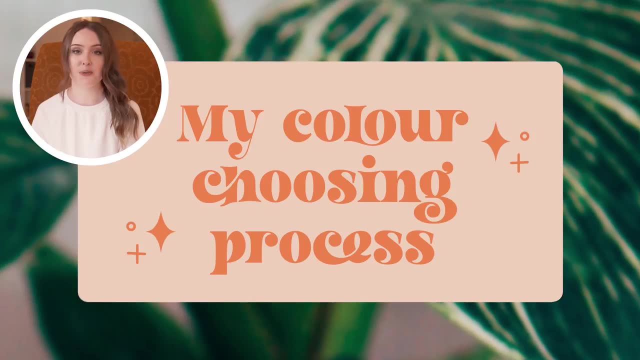 but you can just play around with it and see what you like. Before I finish up, I just want to briefly touch on how I approach choosing colours when I'm creating a new drawing and like where that fits into my illustration workflow, So I usually do it in a few steps. 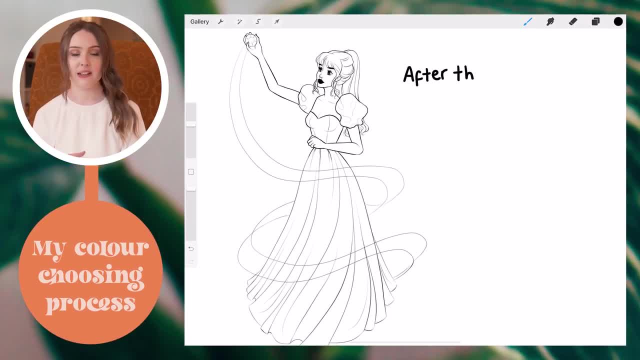 So I typically choose a colour palette when I have completed the line art of my illustration. I may already have like a rough idea of the colours that I want to use before I start, but this is when I do the real like experimenting and refining. 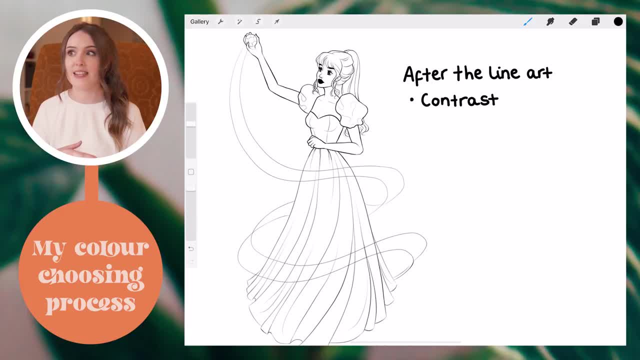 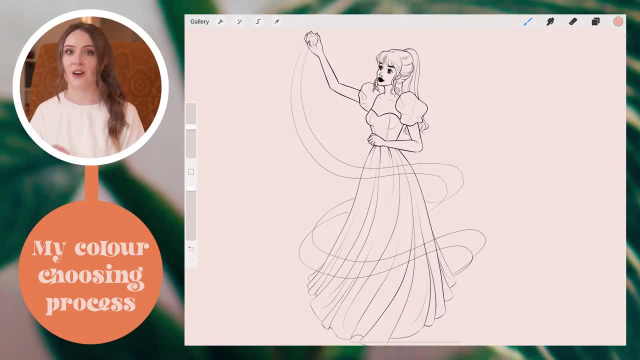 Throughout this process I'm always keeping in mind the contrast and the emotion of what I'm trying to convey in the illustration. I start by setting a background colour and I very roughly block out all the major shapes with a large brush. I try to keep them all on different layers so that they can be altered easily. 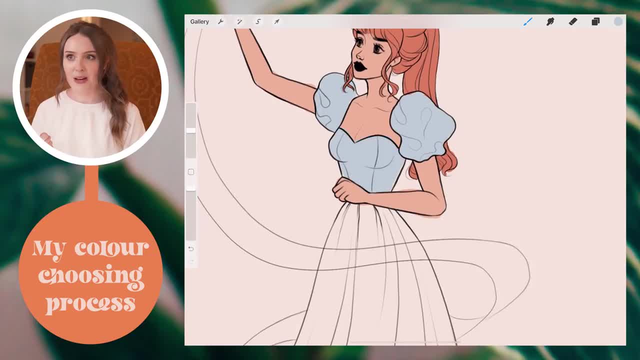 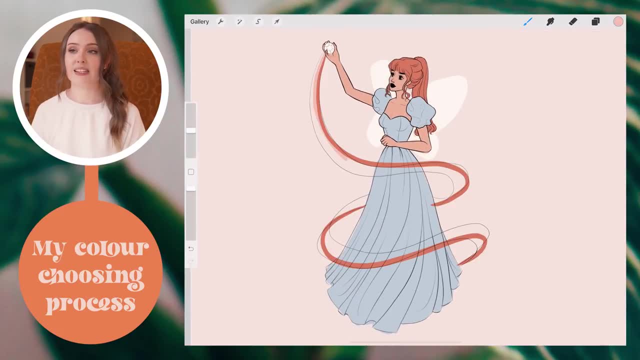 So I usually select the colours in this order: I start with the background and then I do the skin and the hair colour, Then it's clothing and accessories and finally it's the background elements. It's important to choose the background colour first, because this should be the foundation of